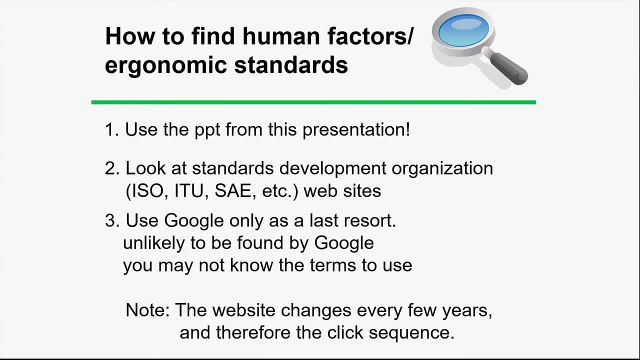 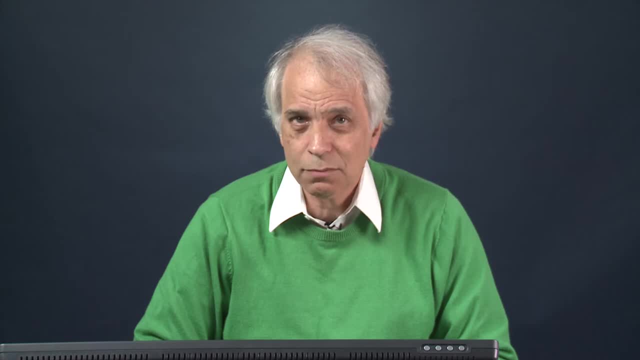 is really a last resort. They don't categorize standards very well. You're not likely to find them without a lot of effort. You may not know the terms to use or how to find them, So I tell people to go to the websites directly, but you need to have some detailed knowledge. 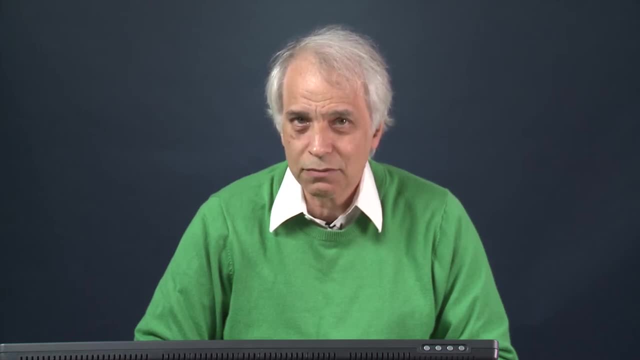 of the organizations involved in order to make that search effective. That's a difficulty. There are commercial organizations that provide standards, categorization and help you search their databases, but often they're for fee organizations and I just don't know a lot of people that actually have used them. 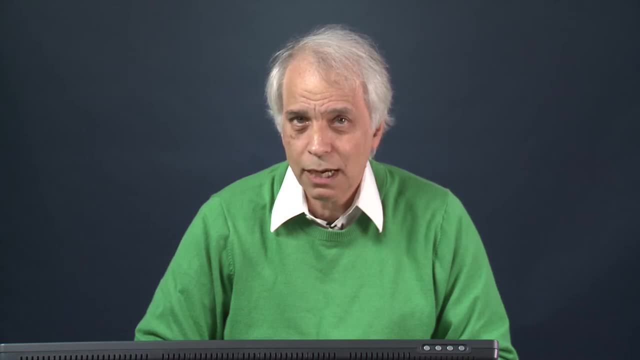 Okay, I'm going to show you how to use them and can give me their personal views on how effective they are. So what I'm going to do next is to show you the ISO website and how to search it. I want to offer a caution: that the website changes every few years, and so the sequence that 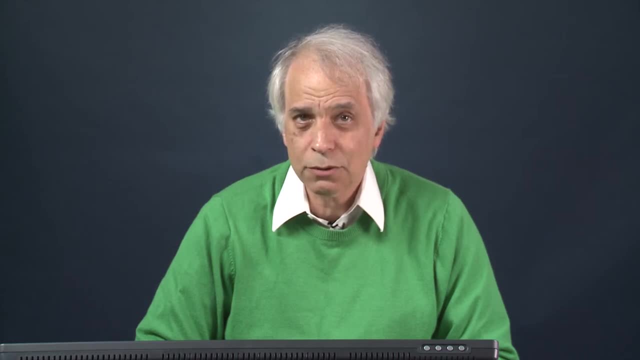 I describe here may not be exactly the way you do it in the future, but the ideas identified will work very well. So at this point, let me break away from the PowerPoints and go to the ISO website. However, for archival purposes, I should comment that the PowerPoint materials will be helpful. 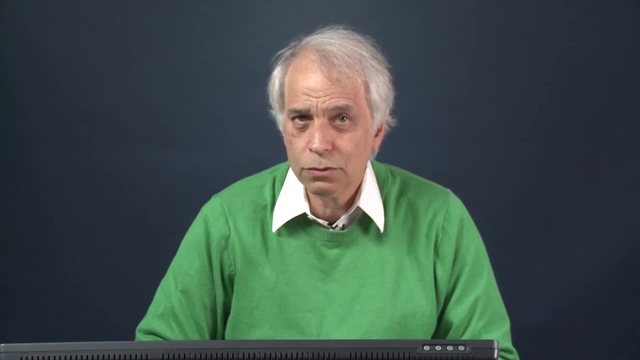 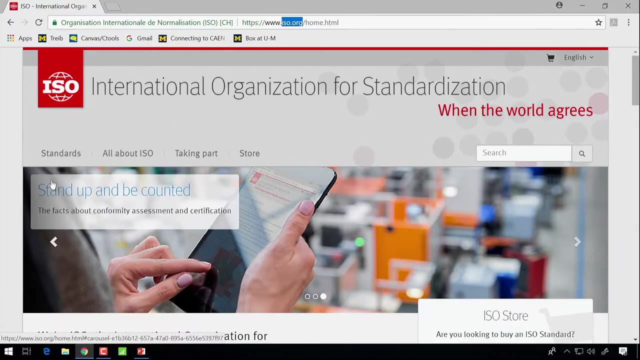 for those that do not have access to this video or prefer to do this presentation on their own rather than using the video. So with that, off to the ISO website. To get to the ISO homepage, one needs to type in isoorg, as shown here, and you can see the homepage for ISO In order to find out about. 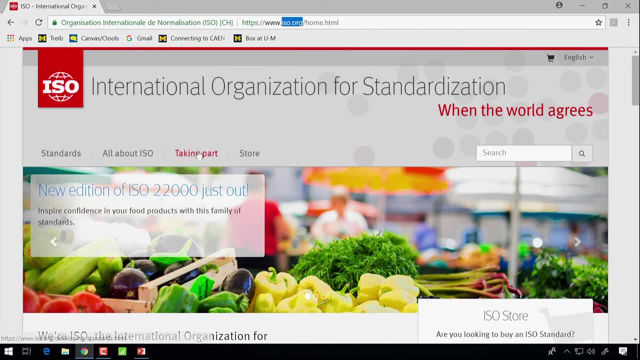 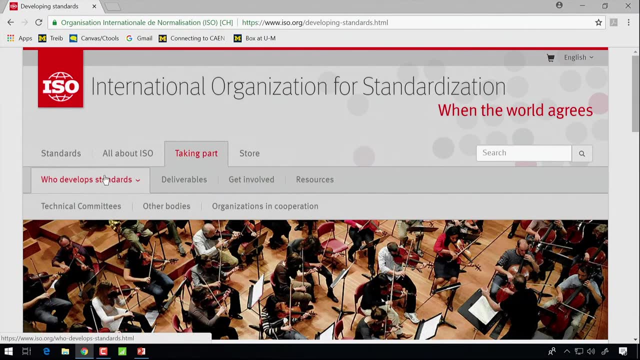 standards. you need to select a particular topic. The first thing you have to do is select Taking Part, and Taking Part takes you down to Who Develops Standards, and below that you want to select Technical Committees. So it's Taking Part- Who Develops Standards, and then Technical. 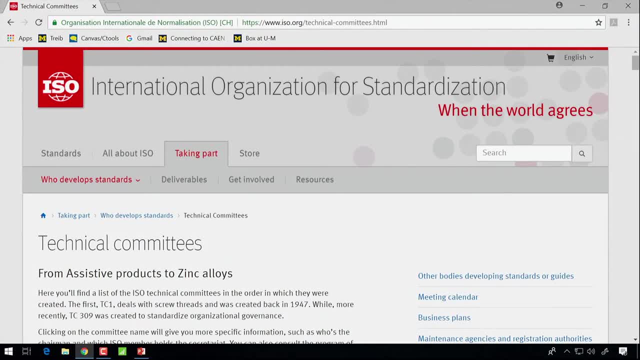 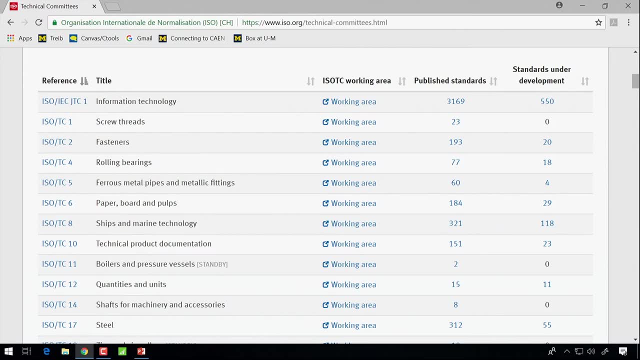 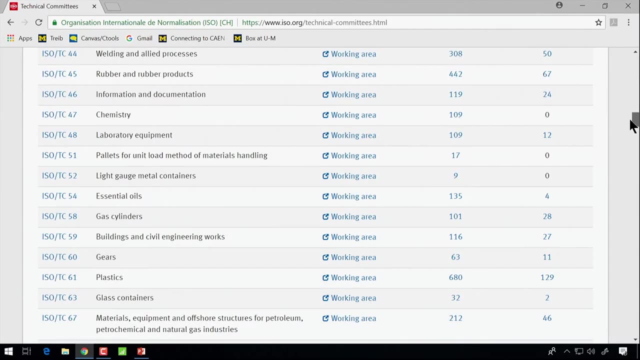 Committees, And what you get when you do that, as shown here, is a list of all the technical committees And, as I had mentioned earlier, there's some 300 of them And you can see the list. I'll just stop and scroll some more and stop and scroll. 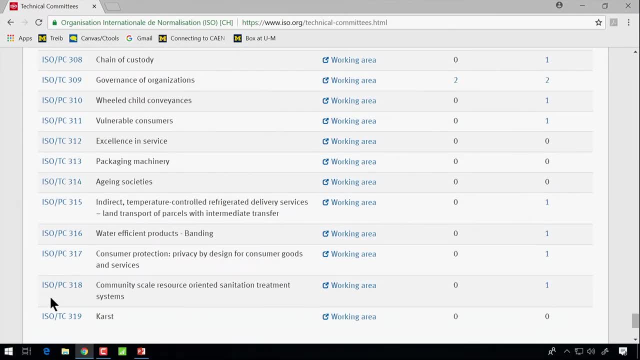 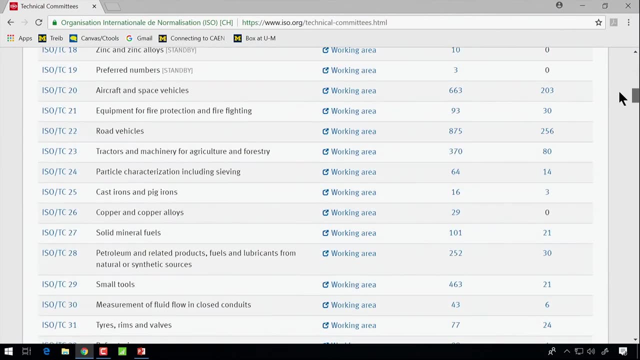 some more And if you go down to the end, you can see there are now 319 committees. For the example that I'm going to provide, I want to focus on ISO Technical Committee 22,, which is road vehicles. So if we click on Technical Committee 22,, we're going to 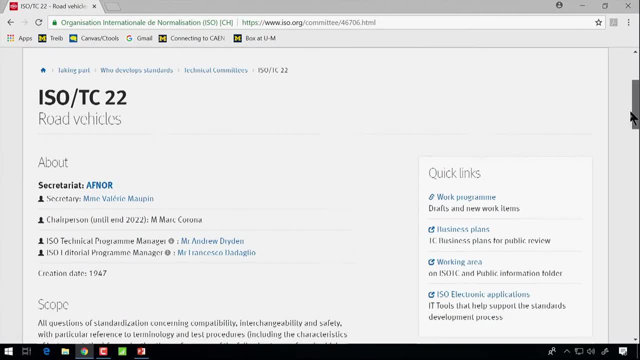 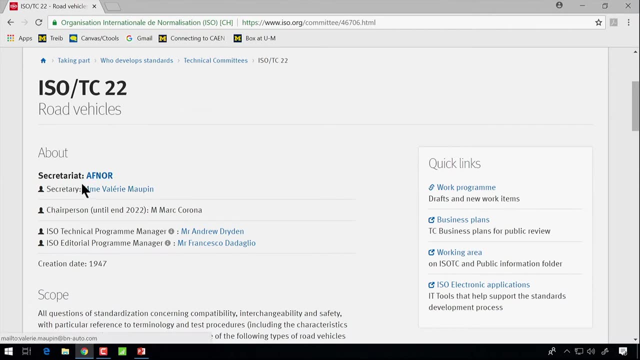 see the list of all the technical committees. So this is a list of all the technical committees. We can see a number of things on their page. So here's a description of the Technical Committee. It's called road vehicles. Here's who the staff people are. Again, this particular Technical 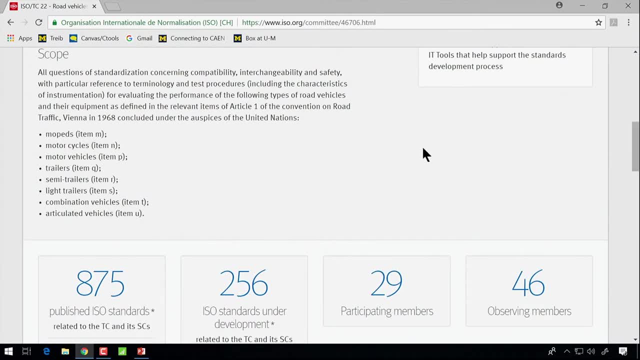 Committee is run by the French Standards Organization, AFNUR. Some other information that's on there is the scope of the committee, the number of standards they have published, which is a huge number- 875,. and the scope of the committee, The number of standards they have published, which is a huge number- 875.. And the number of committees that have been published. Al-Muashef is one of them, and it's 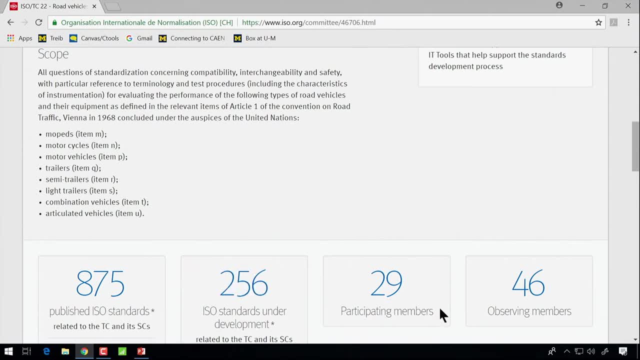 with another 256 under development, and these two items refer to how- how national standards organizations are involved. so there are 29 that are actually participating. they get all the documentation and can vote. the 46 who are observing simply get information but have no ability to vote on standards that are put out by this particular technical committee. 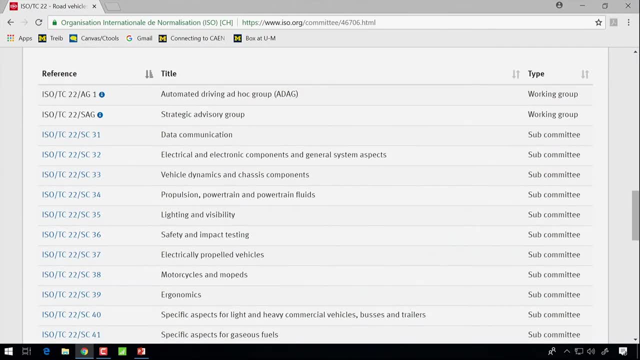 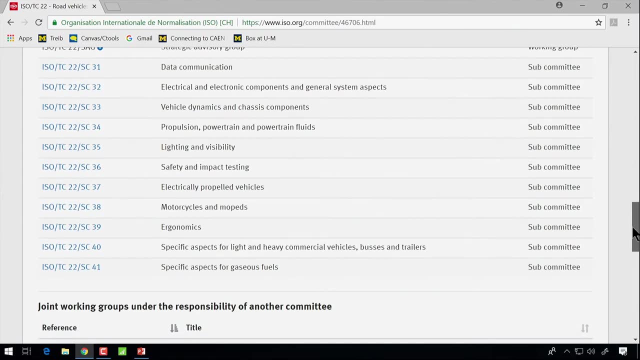 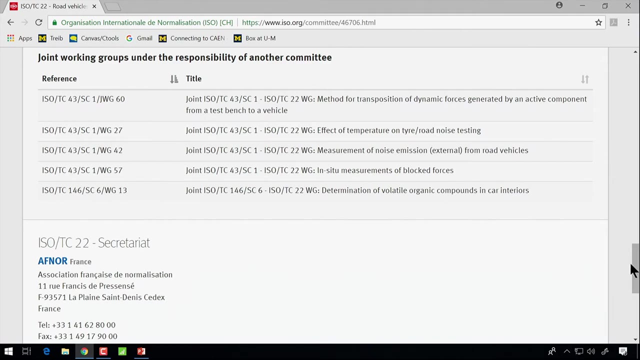 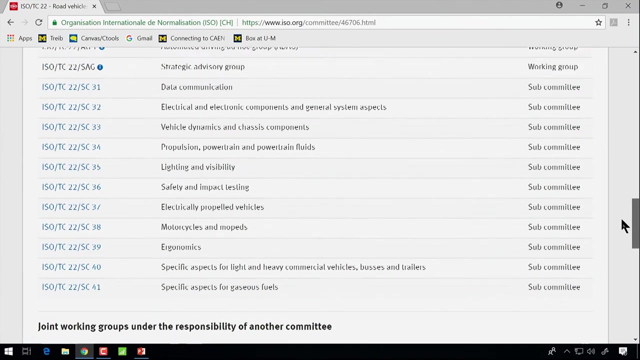 below that are the various groups, the subcommittees, that are associated with this technical committee- and notice there are quite a few of them- and then below that are groups with which they liaison with and finally, at the bottom there's additional contact information for the secretariat. so moving up the technical committee of interest to this particular example is subject. 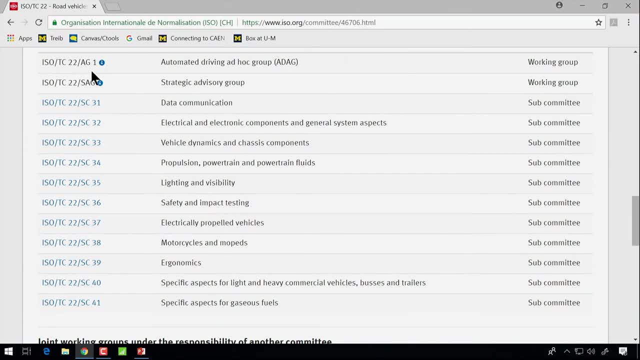 to the technical committee committee 39, ergonomics. If you notice the subcommittees are not numbered from one, and that's because it was some reorganization in the past, so they simply re-numbered the committees to avoid confusion with previous committees they had. So let's look at subcommittee 39, which is ergonomics. Here is their. 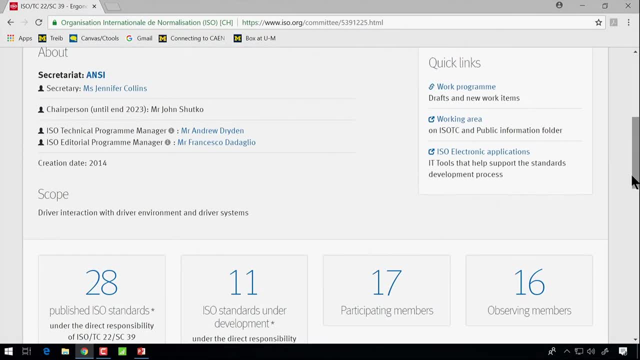 page and if we scroll down you see kind of an interesting aspect to it: that the organization is responsible for this subcommittee is ANSI, the American National Standards Organization. So the technical committee is a responsibility of the French standards organization. This subcommittee is the responsibility. 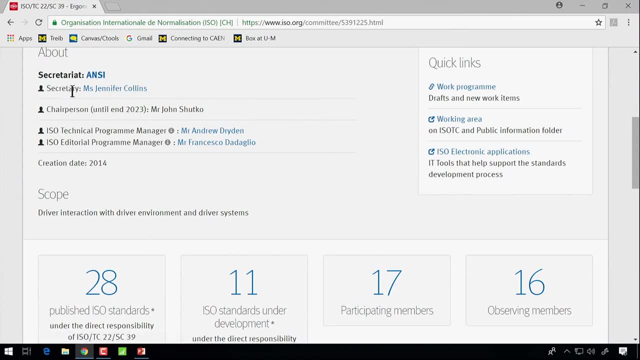 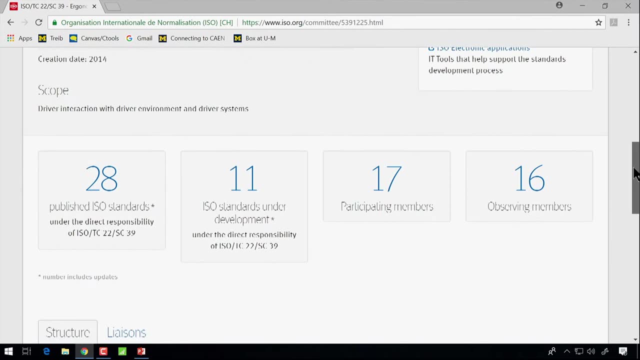 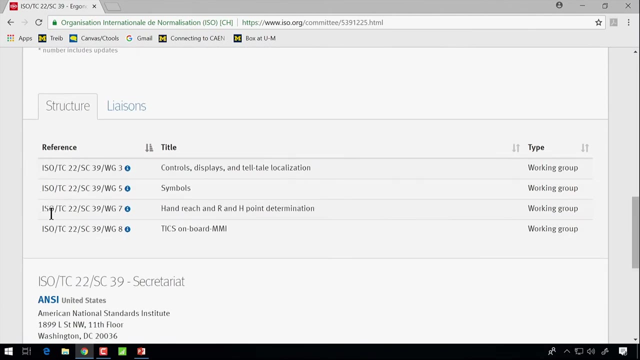 of the American National Standards Institute and in fact they've delegated their activities to the Society of Automotive Engineers. You can see they have 28 standards and they're developing another 11 and they have 11. and they have these following working groups. You can see there are four of them: controls and 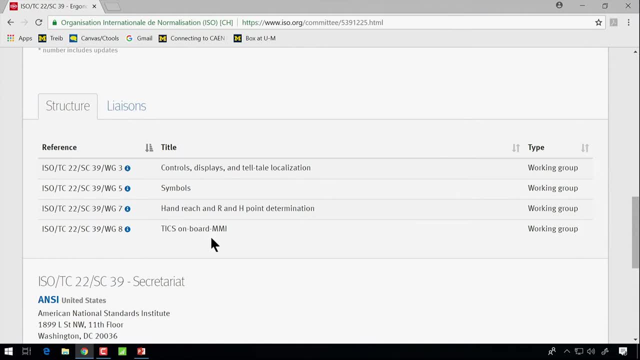 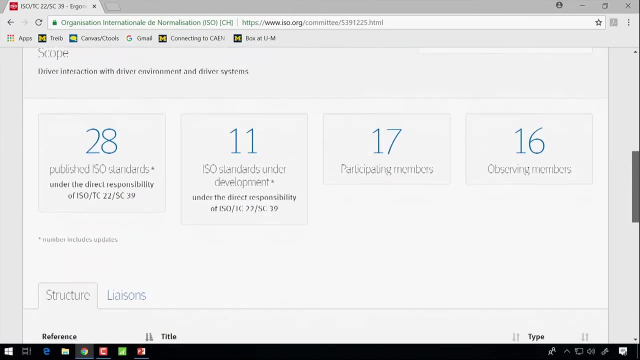 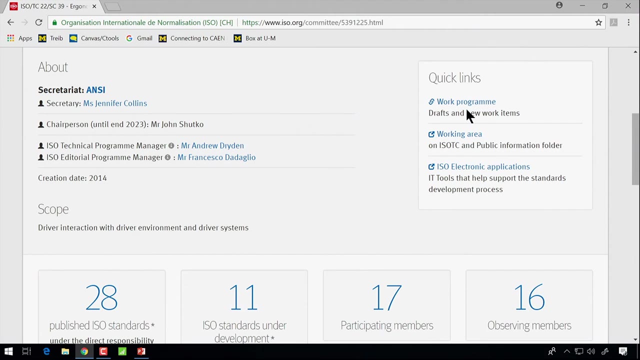 displays, symbols, hand reach and something related to information technology, And here's additional information on contacts. Now, if you want to find out exactly what they're working on, you need to go to their work program as identified here, And if you click on it, up will come information about their 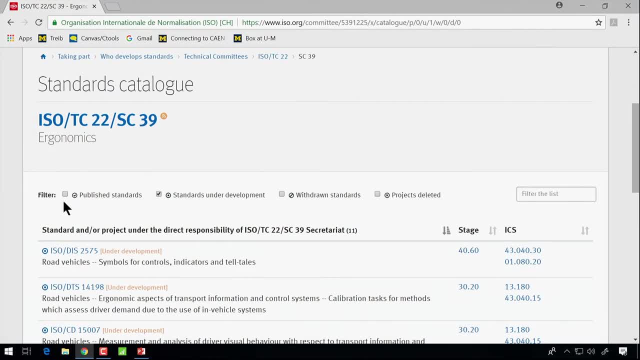 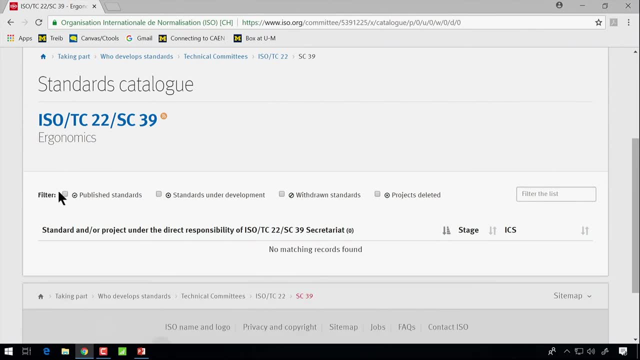 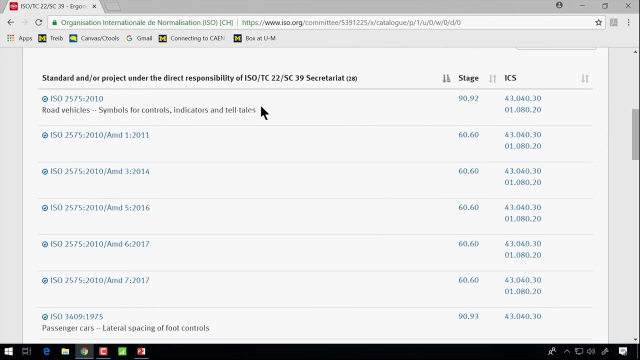 work program And you identify what you want to see by selecting from here. It defaults to standards under development, but what I want to talk about most are standards that are now published. So here's a listing of the standards that are published. So there's a standard. 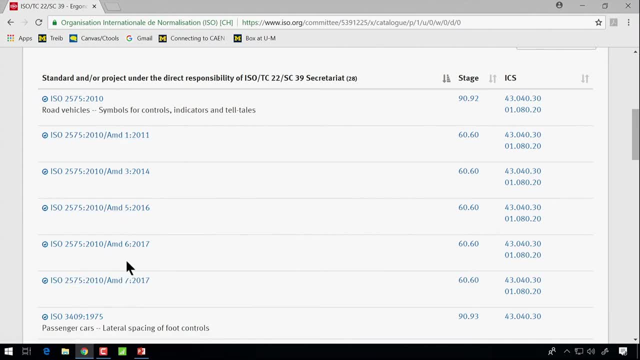 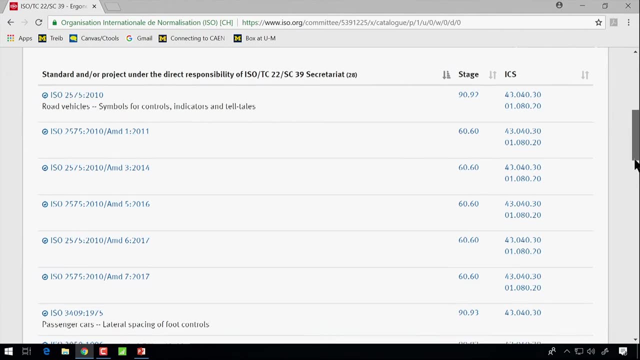 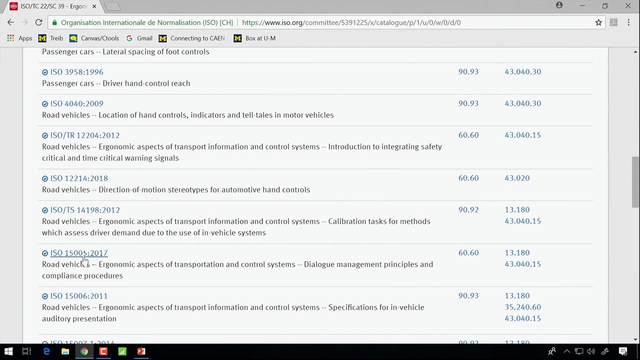 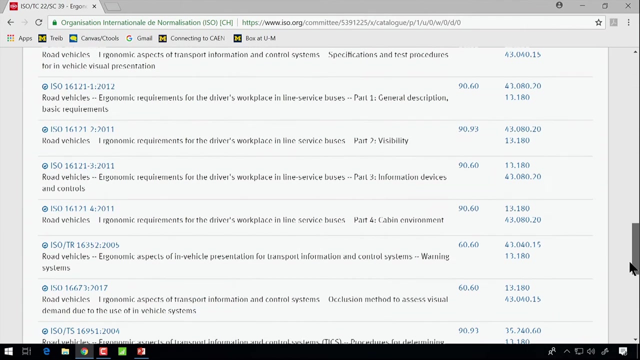 associated with symbols, and each year there's an amendment to that document that comes out, because there's a continual growth in symbols. Here's other standards: foot controls, driver hand reach location, etc. etc. etc. specification for auditory information and so forth. So those of you that are 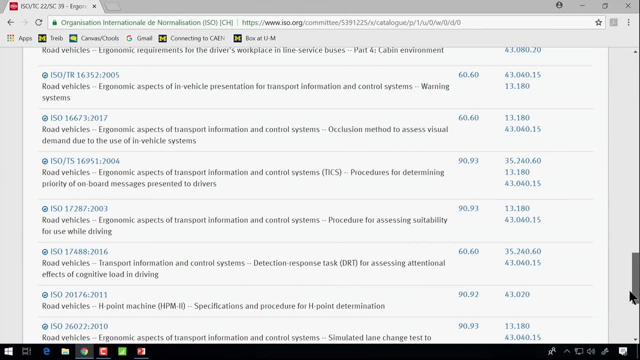 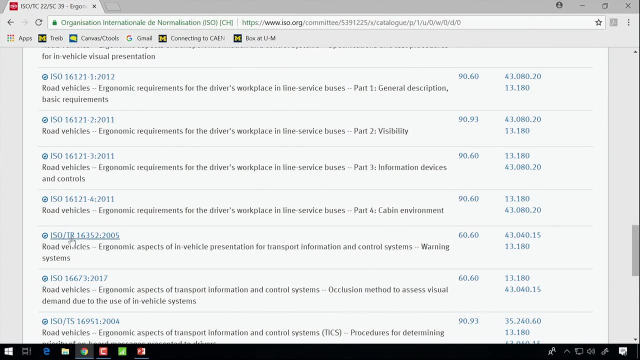 interested in this particular topic can look at these standards at your leisure. Let me just pick one as an example to show you how you can get additional information. So let's imagine we were interested in warning signs. This is a warning sign for warning systems. This turns out to be a technical report. 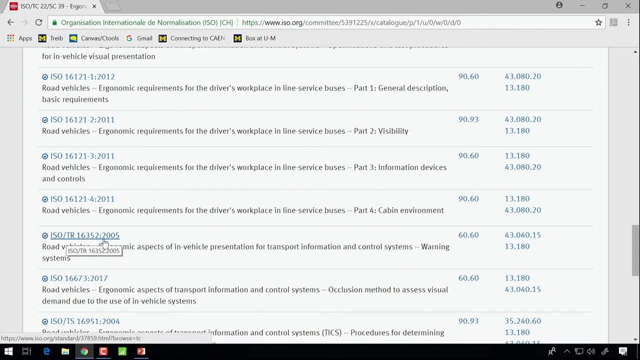 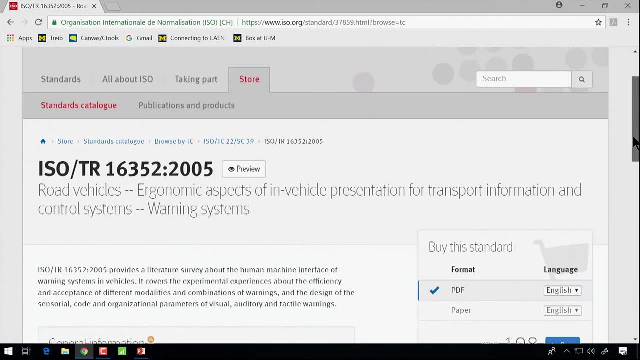 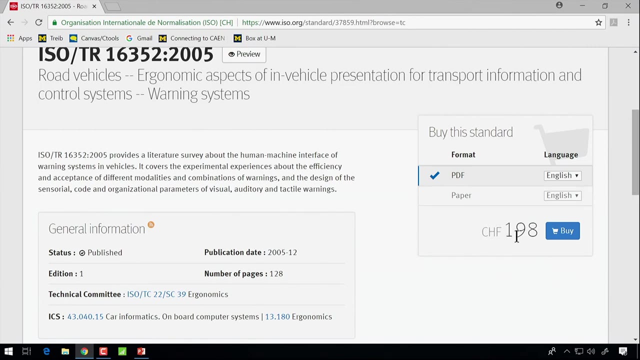 So that's indicated here by TR, So 16352.. Last update was 2005.. So we click on it. We can get information about it. Here it is. Here's a summary of it. There's some additional details right here. The price again: you have to buy these and the 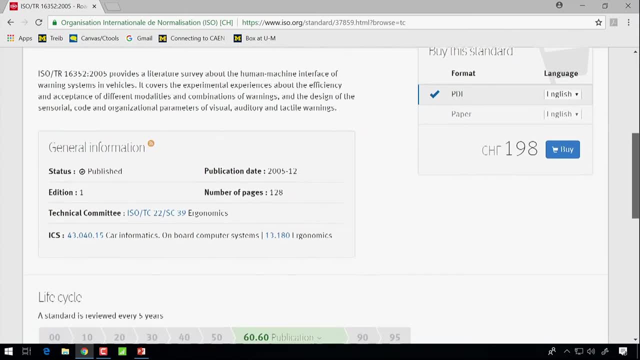 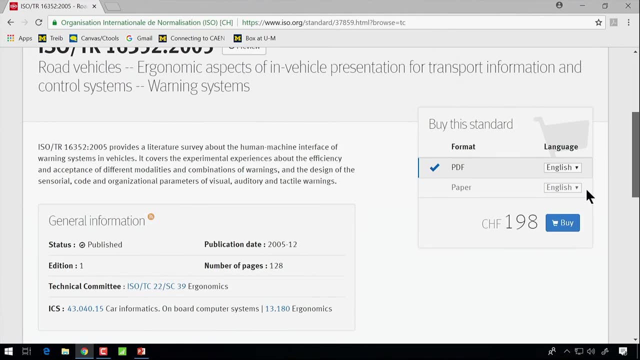 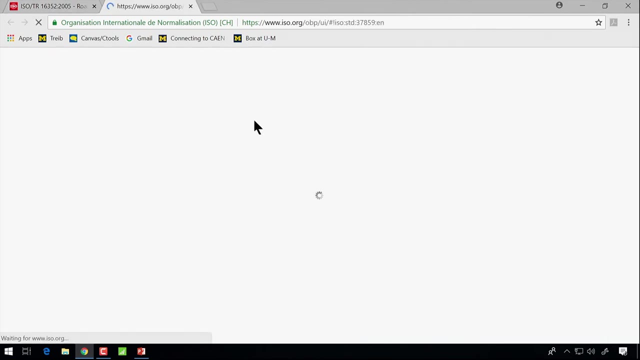 price are in Swiss francs, And then if you want to see it, you can't see so easily. There used to be a way- yes, there is a way- to get a look at it by clicking preview, And then in a moment the preview comes up and I want to say some things about the preview. 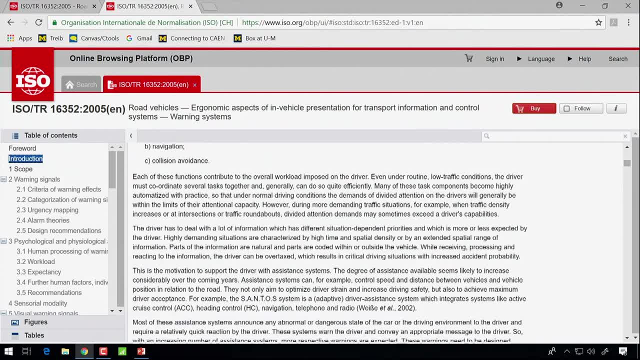 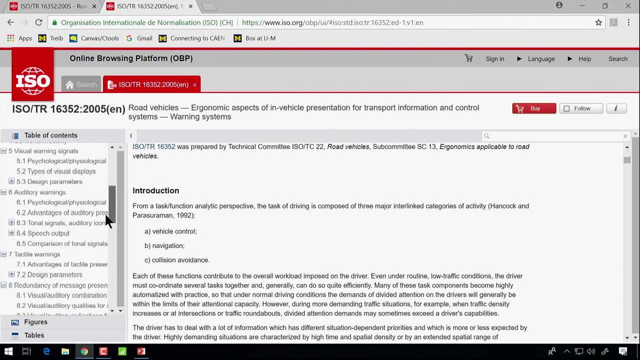 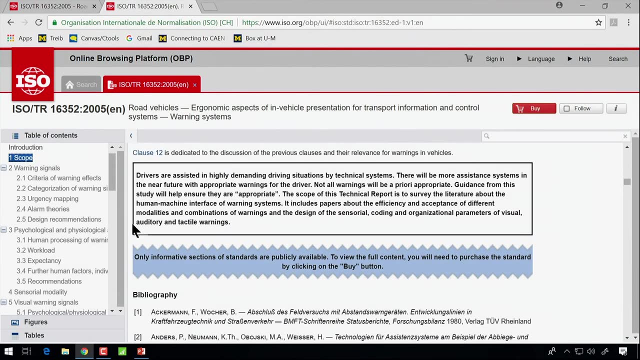 Let's scroll down. So the preview gives you the forward. you get on the left side outline of the document and here you get the scope and you get a bibliography or references, but the bulk of the document is not visible. so if you're not sure, if 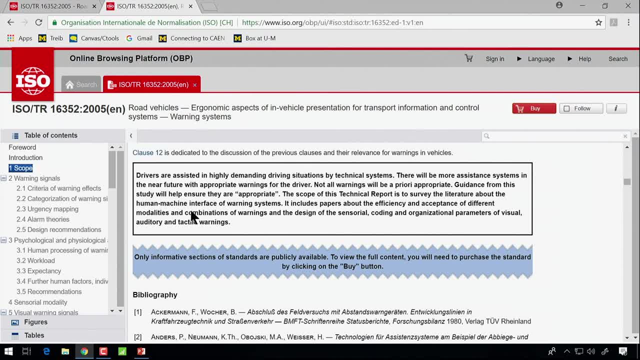 you want it. all you have to make a decision as to whether it's a value to you or not. is this information which is a preview? but the meat of the document is not shown, only introduction definitions and references. so it is a gamble on your part if you don't know what's in it, even though you have some. 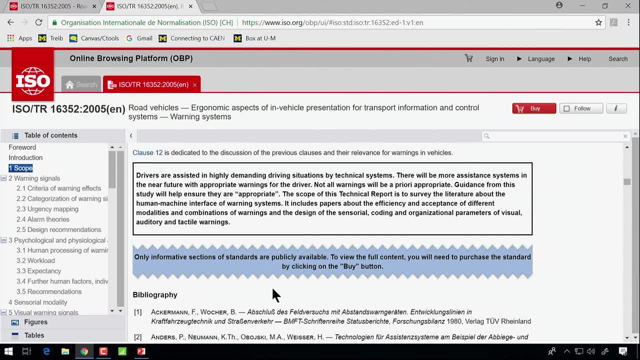 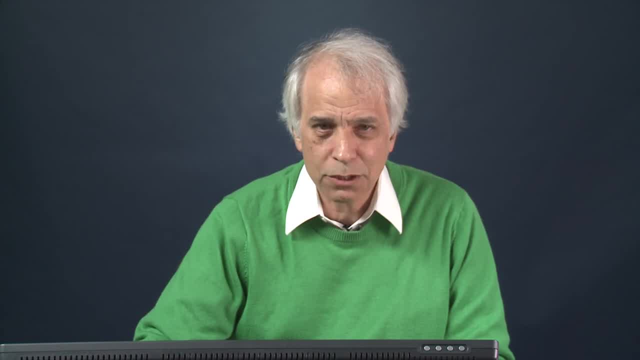 description. there's still a gamble whether that 198 Swiss francs will be well spent or it's not very useful to you. so that gives you a sense of the process by which one finds standards, at least from ISO, and again the process is get down to the technical committee. look at the subcommittees that are associated. 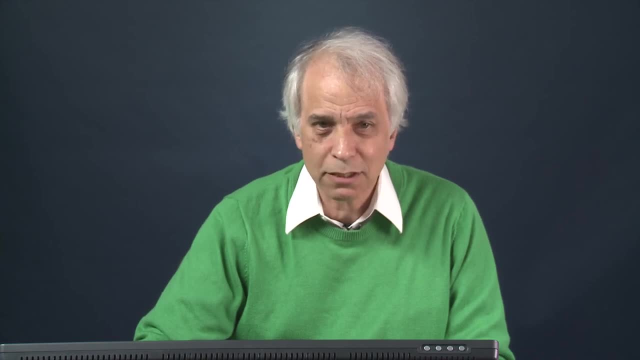 with it, look at their work program. get a look at their work program, get a list of standards and make some decisions about whether what's there is useful or not. other standards organizations- the same process holds. you find the committee that's involved with the work. you see what they're doing and 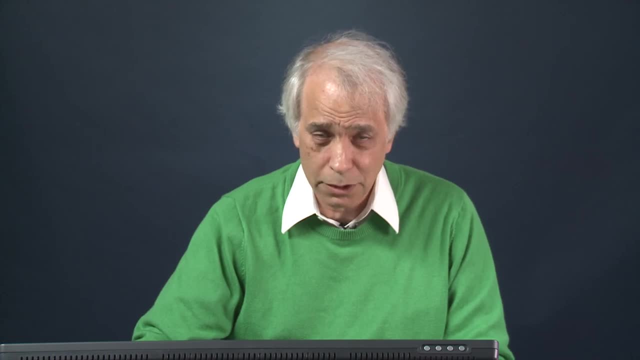 then you try to determine if their work is relevant to what you do or not. one of the alternative strategies is to have somebody in your organization who really knows what's happening in standards and to ask them for guidance. involvement really makes this process a lot easier. again, the strategy you'd like to do is to go to Google or some free public. 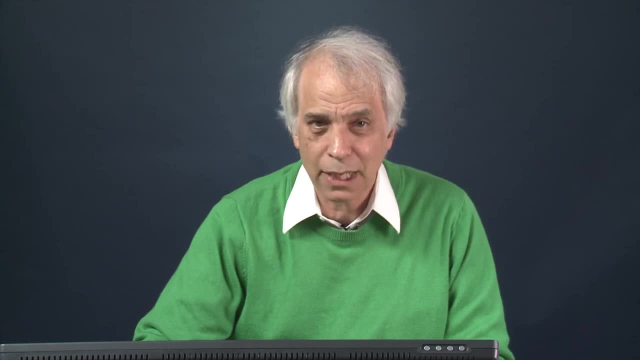 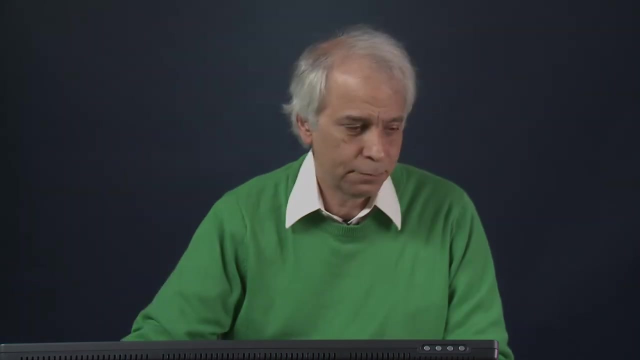 database, be able to get access to the standard by typing in some names and then download it, and that just doesn't happen. so hopefully that's helpful to you. and now we'll move on to the third part, which is looking at specific human factors and ergonomic standards in detail.